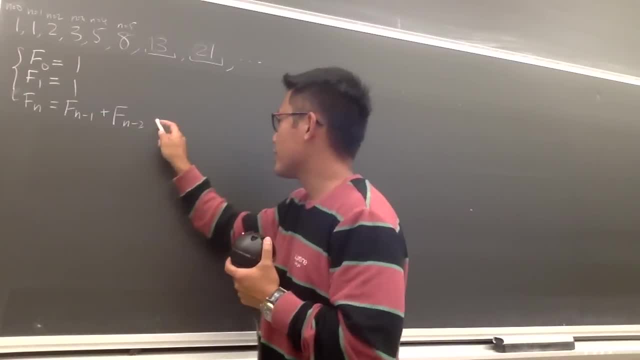 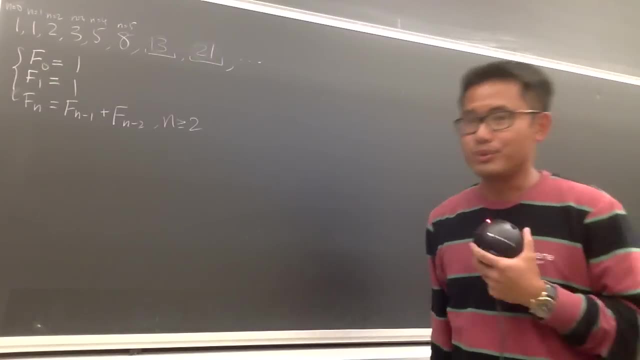 Anyway, this is the recursive formula alright, And technically I should say this is only legit when n is greater than or equal to 2.. So that's pretty easy to do right. But the trouble for a recursive formula is that what if I want to figure out f of 100?? 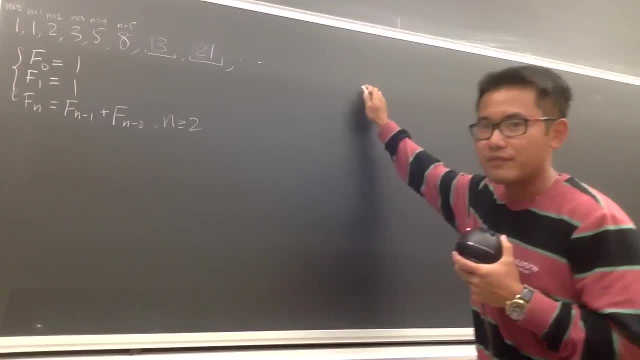 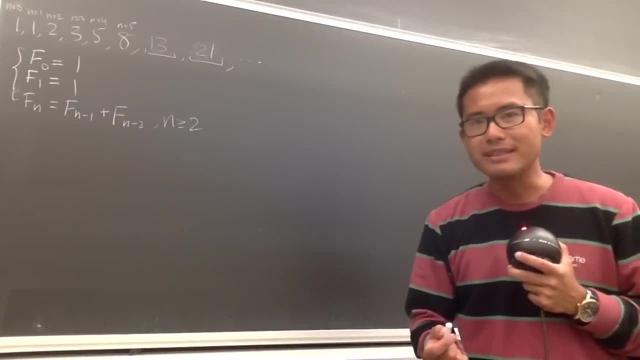 In order for us to figure out f of 100, we have to figure out f of 99 and 98. That's not fun, right? So I will show you guys how to find the n's term formula, right? So just explicit formula based on n only. 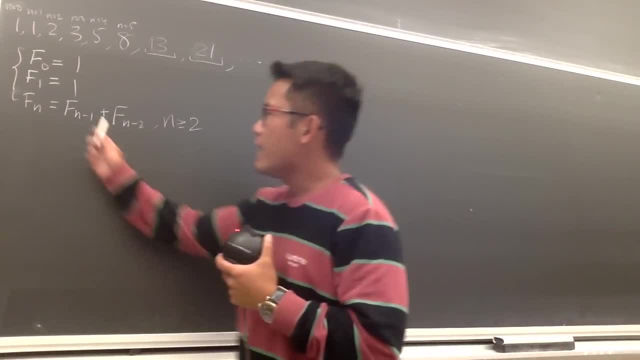 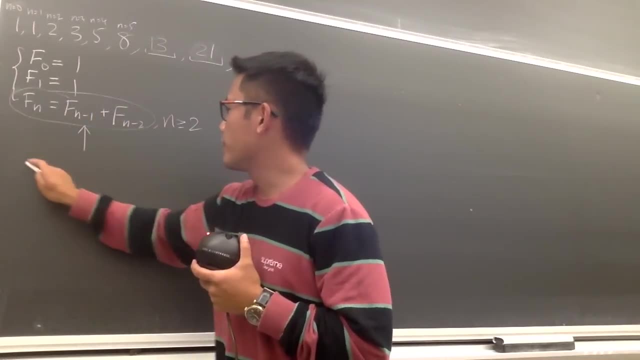 And this is how we are going to do it. Whenever you have this kind of formula right here, we'll just call this to be a formula. for now, This right here is what we call the difference, So I have to spell it out. 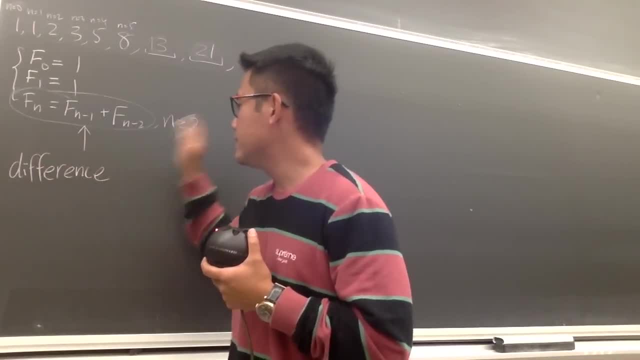 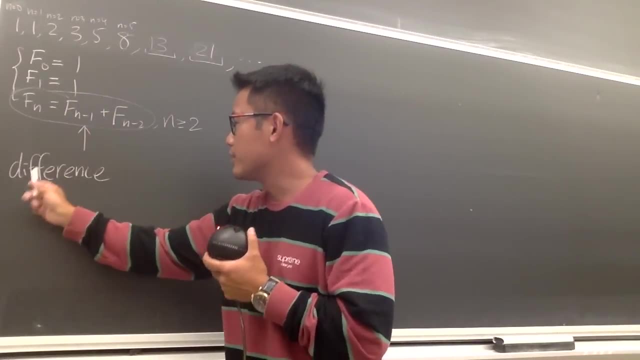 So I have to spell it out: D-I-F-F-E-R-E-N-C-E this time, because sometimes they put D-I-F-F stands for differentiation or whatsoever, right? Anyway, this right here is called the difference equation. alright, It's very similar to differential equation. 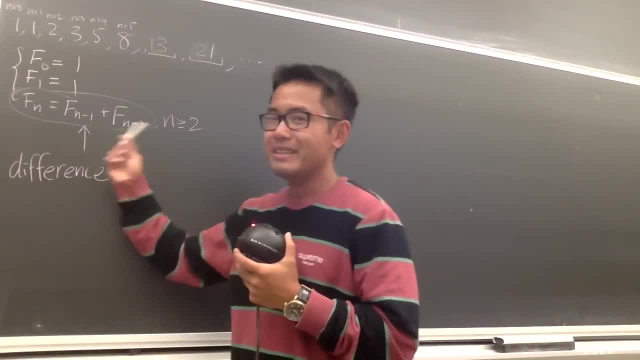 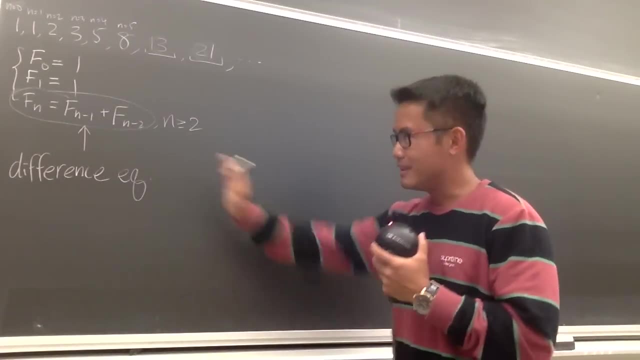 This right here. I will call this to be the second order, Very similar to the second order linear differential equation. alright, This is the second order difference equation And to do this right here, it's also very similar to how to solve the second order linear differential equation. 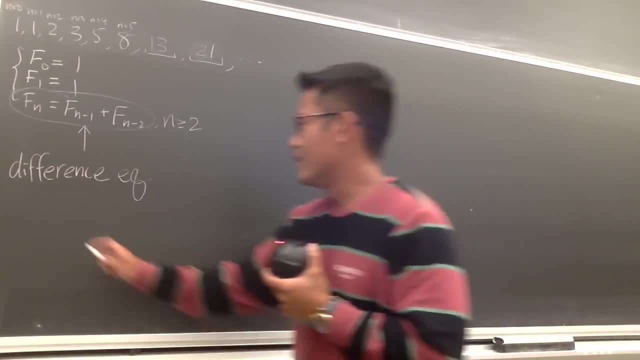 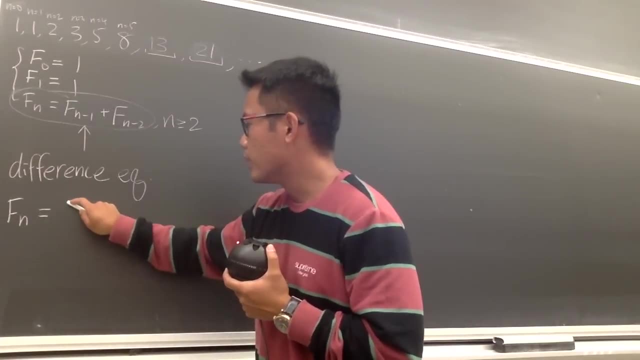 But once again, this is a difference equation. Anyway, to do this, what I'm going to do is that F of n- right. The general form we're going to use is: F of n is equal to some number, R to the n's power right. 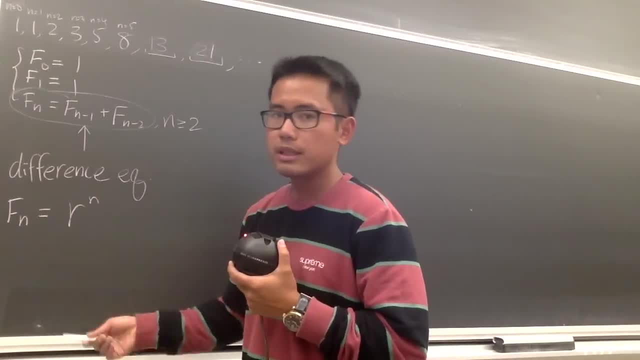 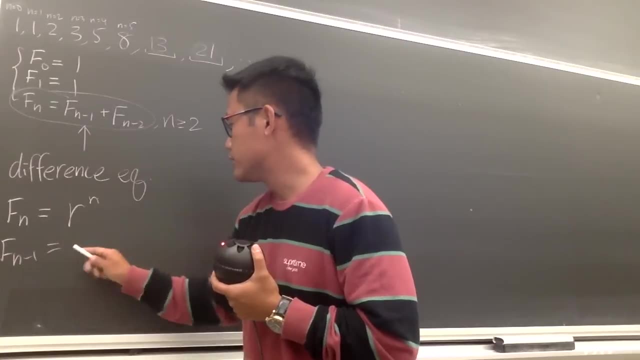 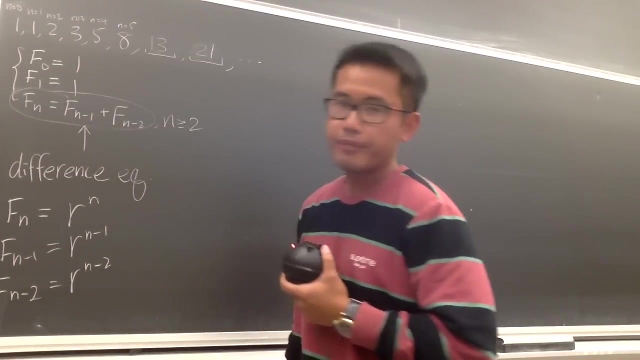 So this is the idea, And what we'll do is, if you know, F of n is equal to R to this sum and value F of n minus 1, this is just going to be R? n minus 1, and then F of n minus 2 is equal to R n minus 2.. 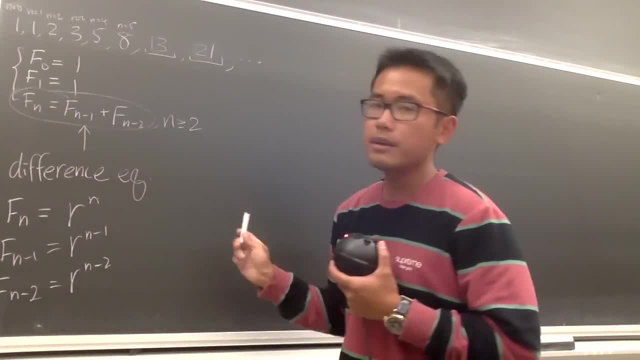 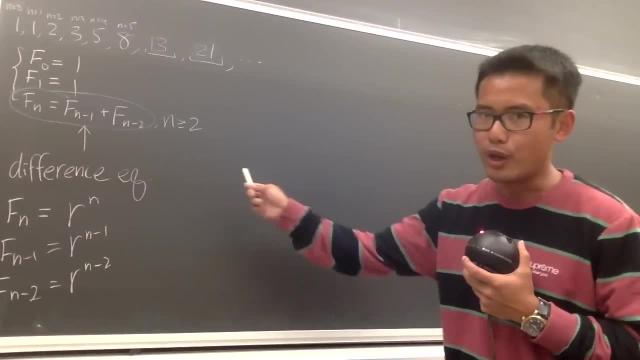 And the deal is that we're plugging all this right here into this equation and we'll have to figure out what R is equal to, And if we end up with two different R values- and in fact we will- we are going to set it up accordingly, alright. 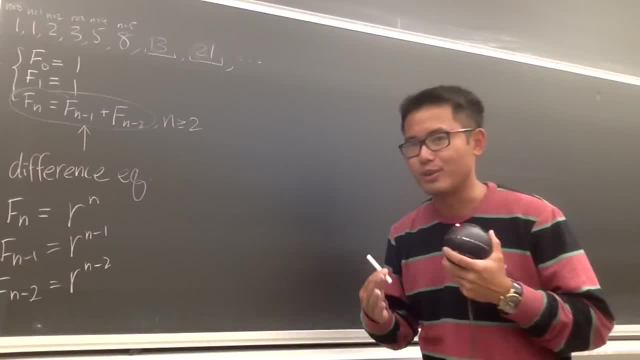 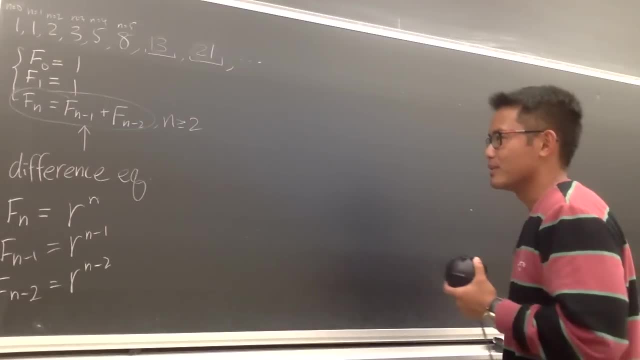 But I'm not going to get into this in too much detail. I'll just show you guys how this is going to work And I will do more If you guys comment down below if you are interested to see how to solve difference equations. 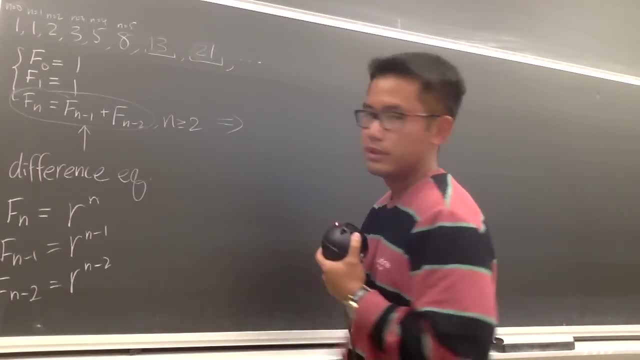 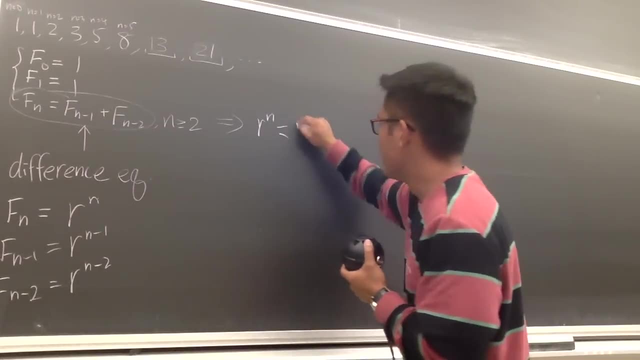 Anyway. so here we go. I'll just put it down right here: F of n is R to the n's power, and then F of n minus 1. is that So R n minus 1 plus R n minus 2? for that as well, right? 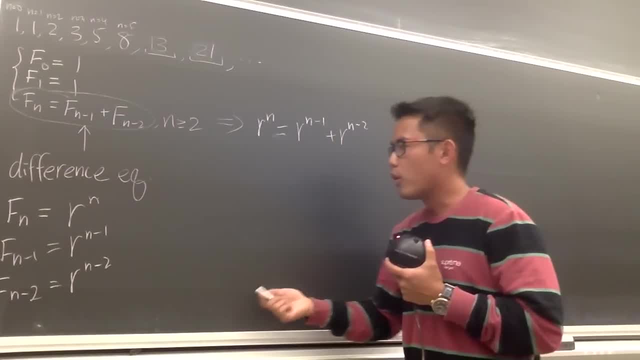 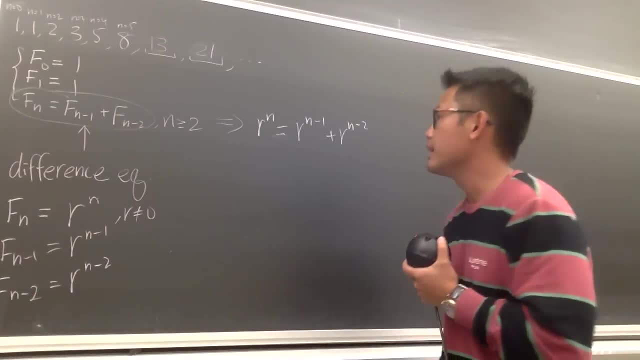 And right here, what we can do is, of course, we don't want R to be 0. Otherwise, if R is 0, that's redundant. R cannot be 0 in our case, right? So what we can do is we can divide everything by R to the n, R to the n, R to the n. 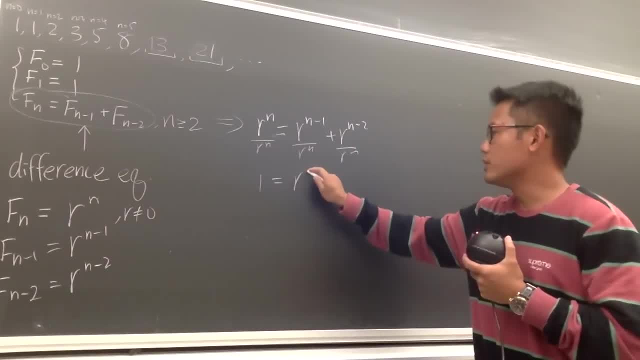 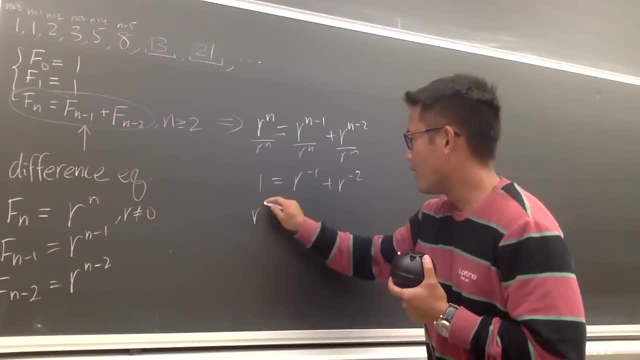 and then we're left with 1 equals to you. do this: If you're watching the video, you can see this right away. right, And then I will multiply R squared on both sides So you will have R squared equals to R, to the positive first power, plus 1.. 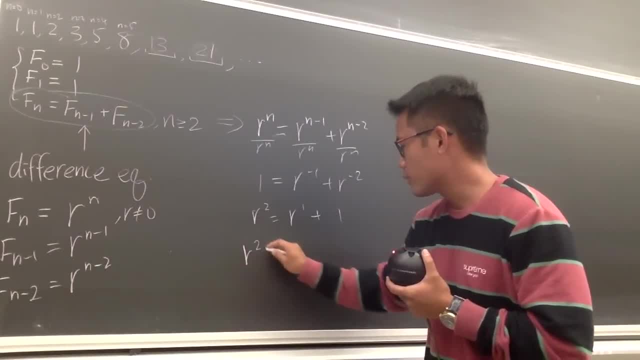 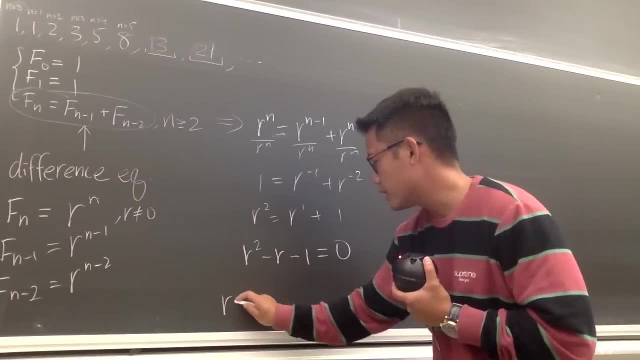 Put all this to the right-hand side. So left-hand side means so you have R squared minus R, minus 1, equal to 0.. And I'm going to solve for R right here, So I will use the quadratic formula. R is equal to negative B, which is negative 1, right here. 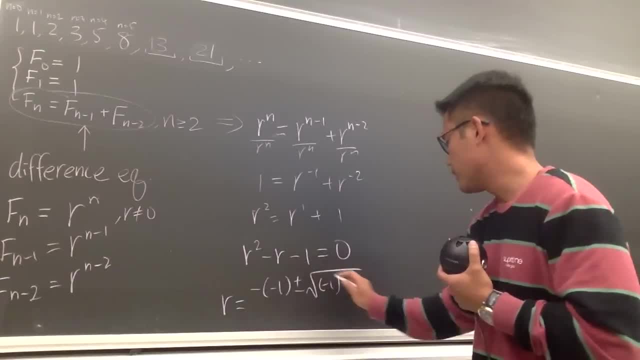 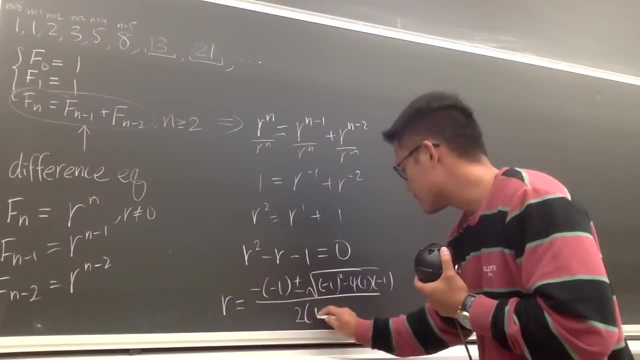 plus minus square root of negative 1.. For the B-value: square minus 4.. A is 1, C is negative 1.. So it's going to be like this: All over 2 times A-value, which is 1, right. 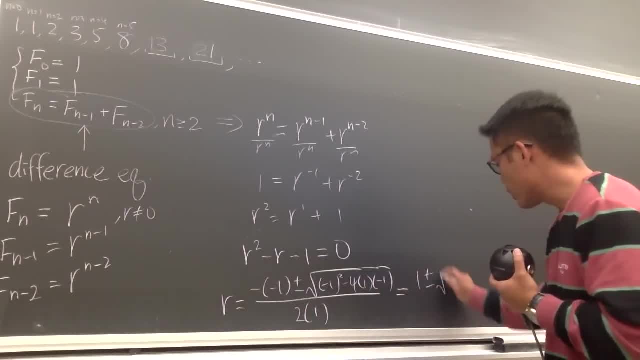 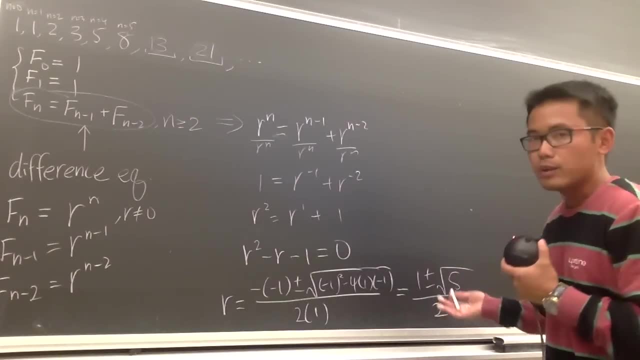 And then you do this, you do that. The first one is just 1 plus minus square root. of all together, inside it's going to be 5, all over 2 times 1, which is 2.. Okay, so you see, we end up with two different R-values. 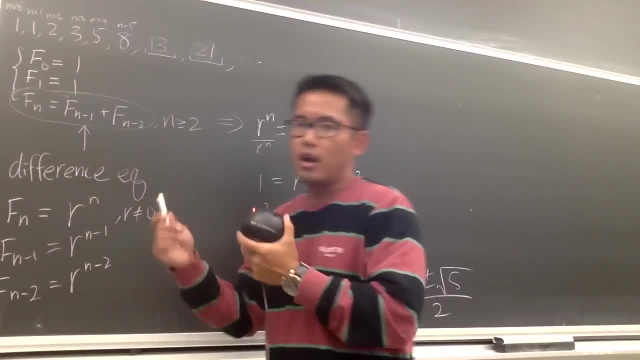 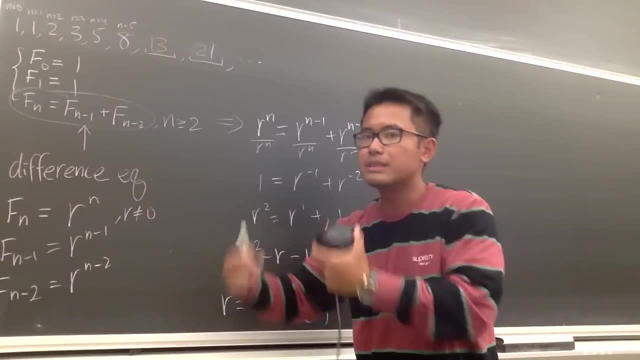 And you know beforehand because you have two of these R minus 1 and R minus sorry, F of N minus 1, F of N minus 2.. So the F of N minus 2 is the previous previous term, just like the second derivative, that idea, okay. 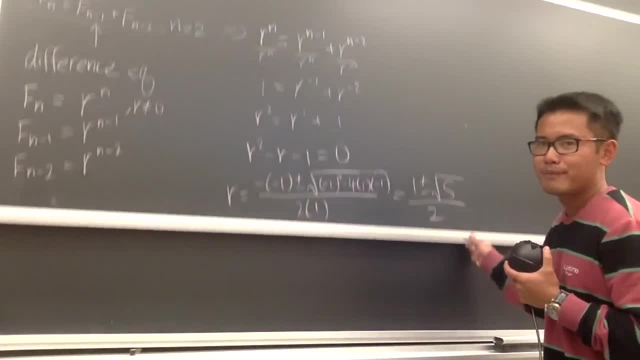 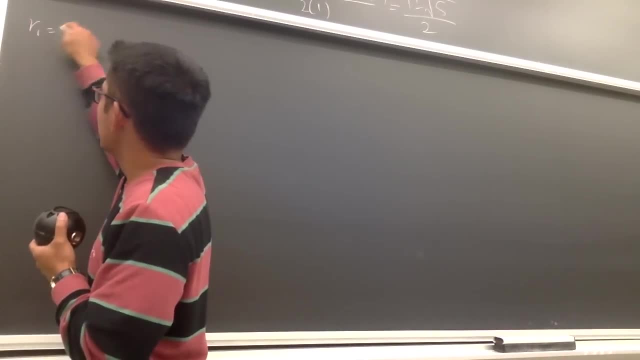 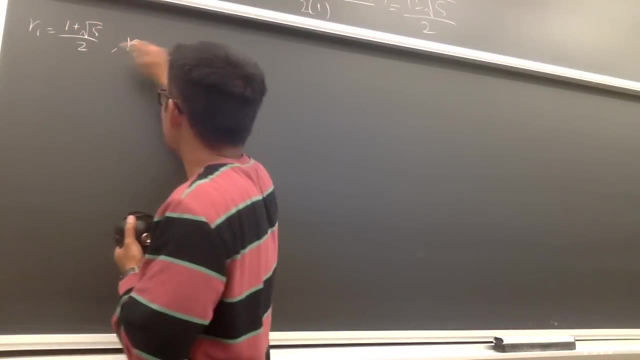 But anyway, we have these two R-values right. So I already done right here for you guys. R1 is equal to- let's put on the positive version- 1 plus square root of 5 over 2.. And then R2 is equal to 1 minus square root of 5 over 2, right? 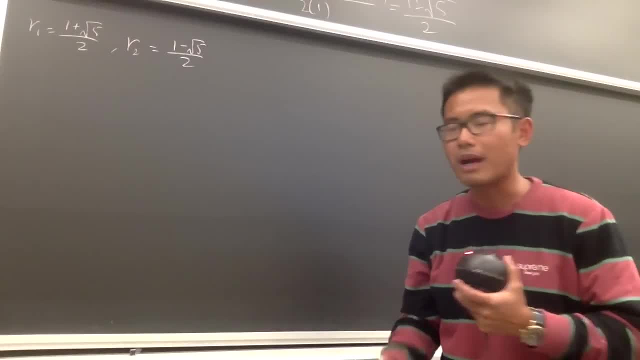 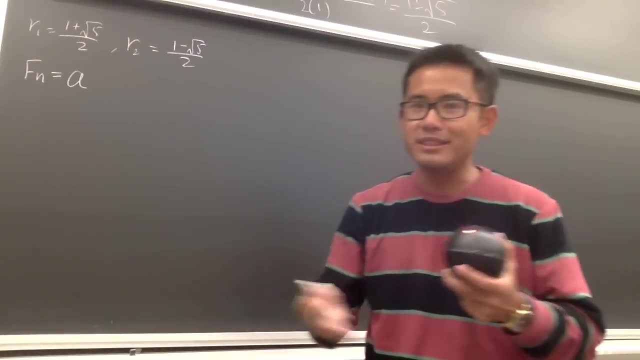 And now this is how we are going to put together and then come up with the formula. Here F of N is going to be some number A. It's just like the C1, C2 whatsoever in our differential equation. But let me just use A. 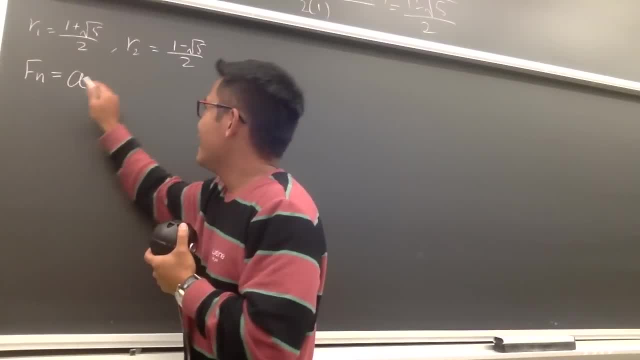 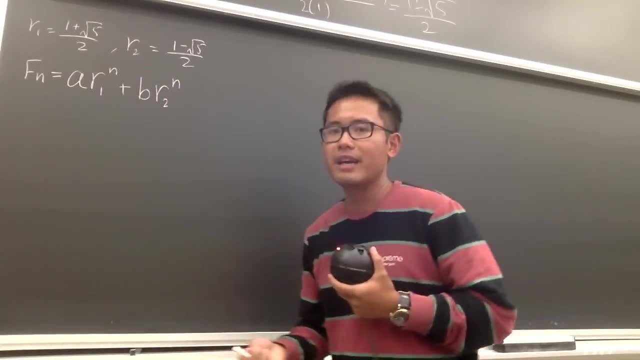 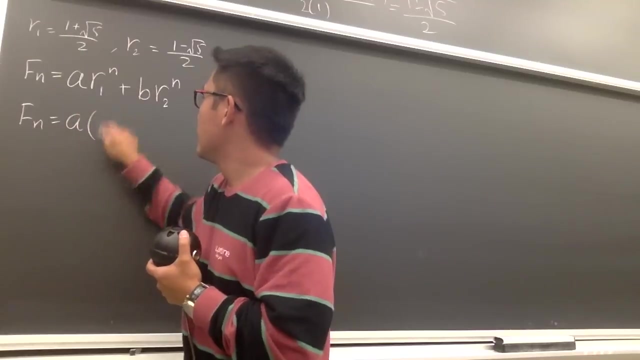 because I like it better. in my opinion, A times R1 to the Nth power, plus B times R2 to the Nth power, And once again we have two different R-values and we just put them together. So FN is going to be A R1, is that? 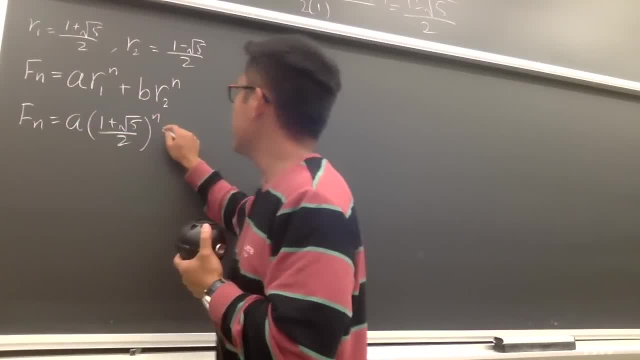 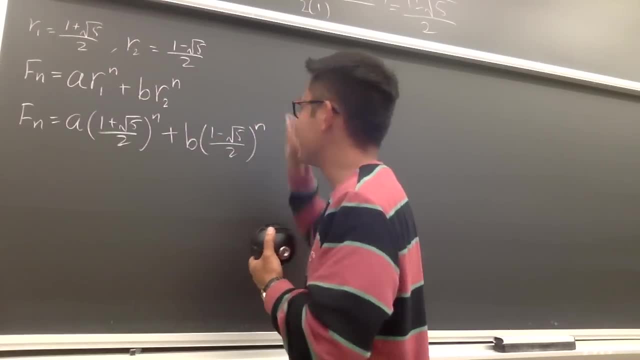 1 plus square root of 5 over 2 to the N plus B. times that 1 minus square root of 5 over 2 to the Nth value, right, Okay? so, if you would like, this is how we are going to solve for A and B. 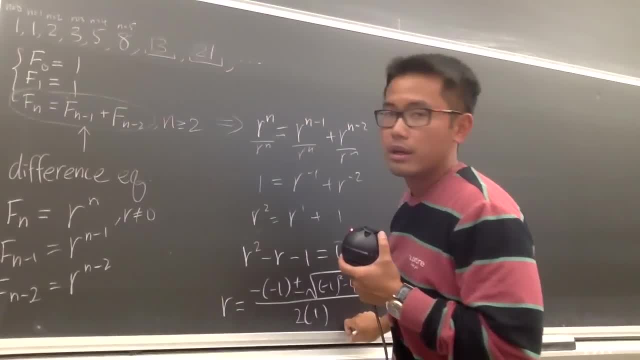 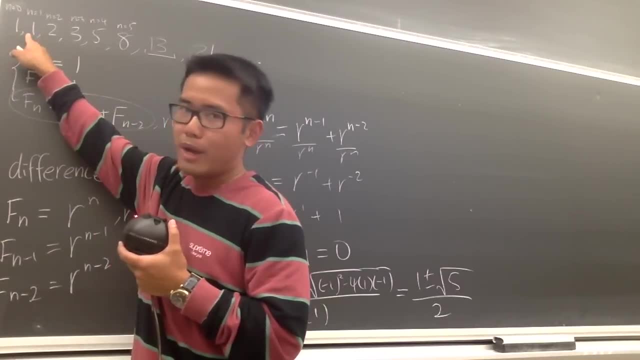 If we can do that, we are done. So here's the deal, As you see: when N is equal to 0, we have 1.. When N is equal to 1, we have 1.. We are going to pick the first two conditions. 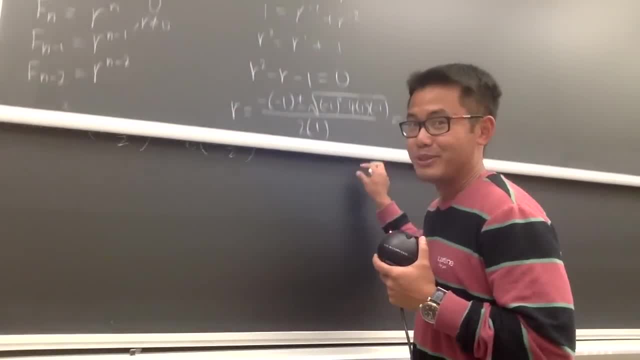 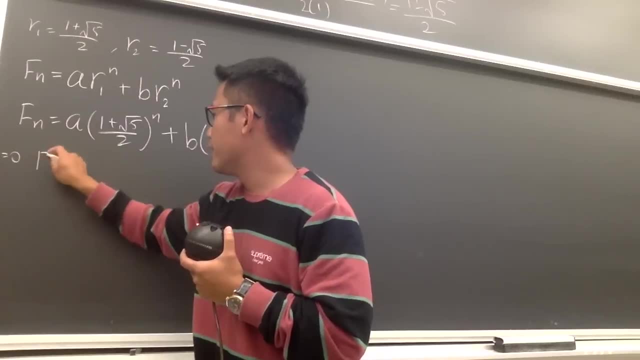 and we can solve for A and B, right? This is really cool, isn't it? So I will just write this down: When N is equal to 0, we know F1, which is sorry. F0 is 1,. 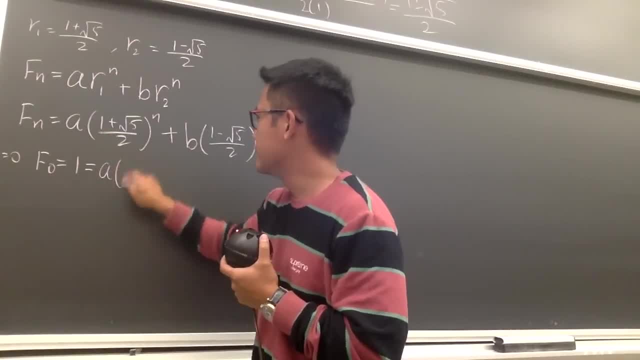 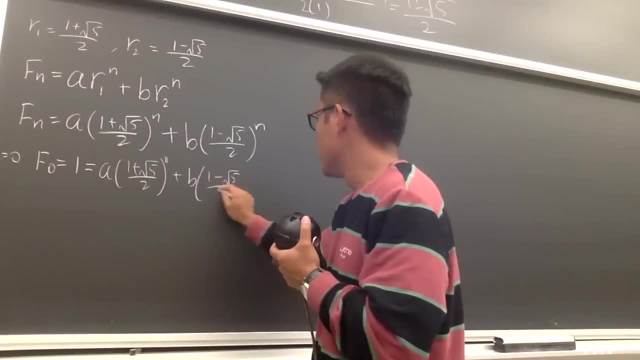 and in that case you have A times this: 1 plus square root of 5 over 2 to the 0th power, plus B times 1 minus square root of 5 over 2 to the 0th power, right. 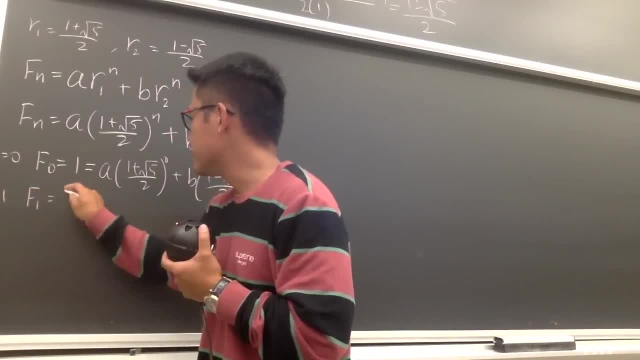 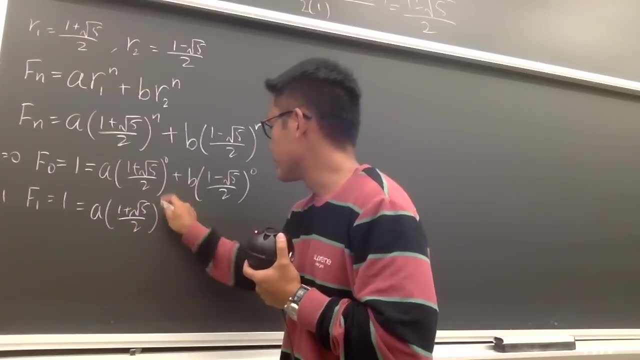 And likewise, when N is equal to 1,, you have F of 1,, which is also equal to 1.. And then you just have A 1 plus square root of 5 over 2 to the 1st power. 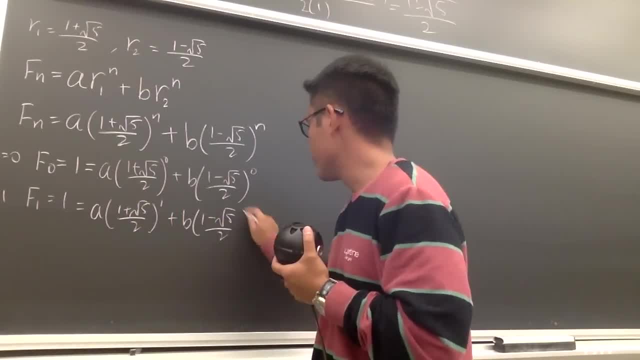 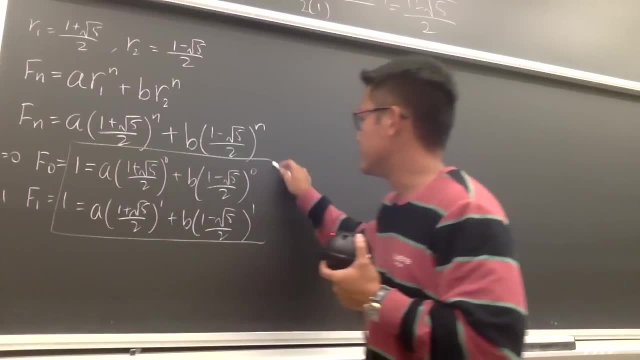 plus B, 1 minus square root of 5, over 2 to the 1st power, just like that. Okay, as you can see, right here, we have a system of equations in terms of A and B. If we can solve for A and B, we are done. 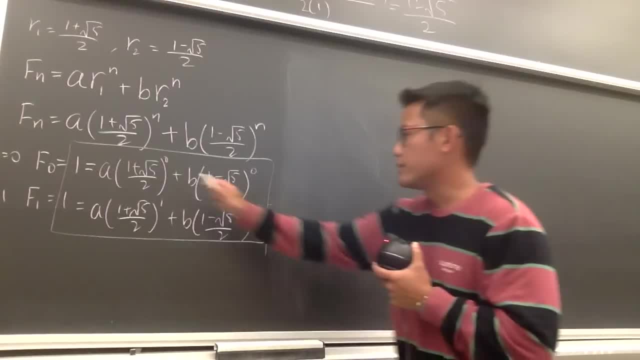 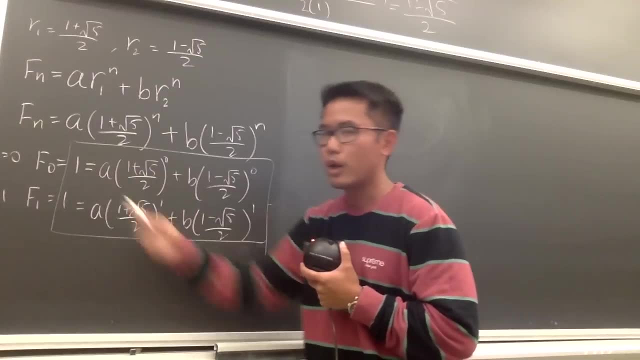 And I wanted to solve this by elimination method. So if you look at the first equation, we know this is just going to be 1, and likewise this is going to be 1 as well. So all in all, we have A plus B is equal to 1, right. 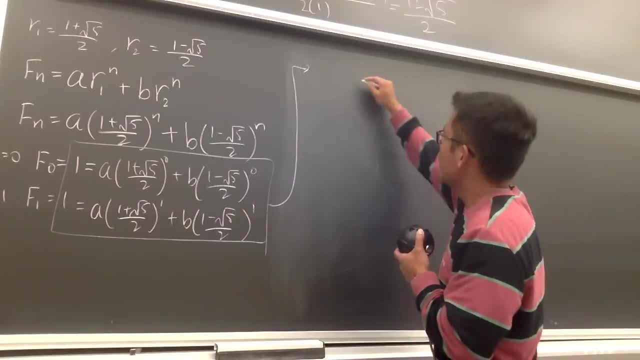 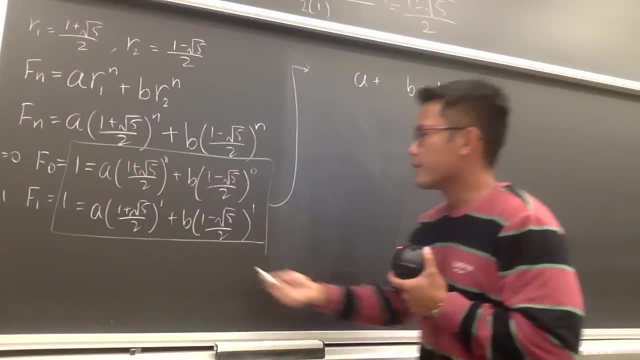 And let me just write this down again. First equation: we will have A plus B equals to 1. And let me put it down like this, right. And then for the second equation, we just have to deal with these two numbers. 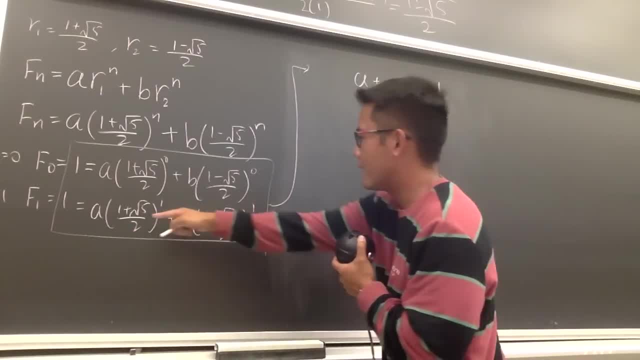 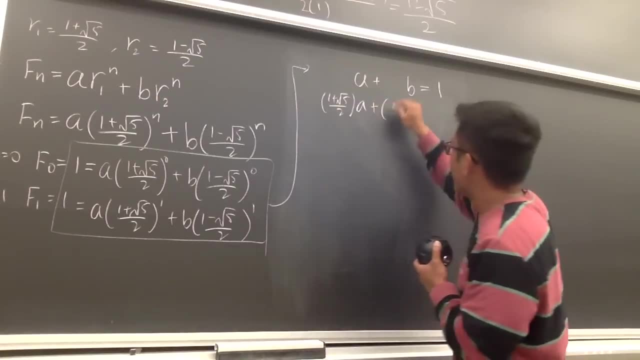 And let me put down these numbers in front right. So we will have that which is 1 plus square root of 5 over 2 times A, and then this is plus 1 minus square root of 5 over 2 times B. 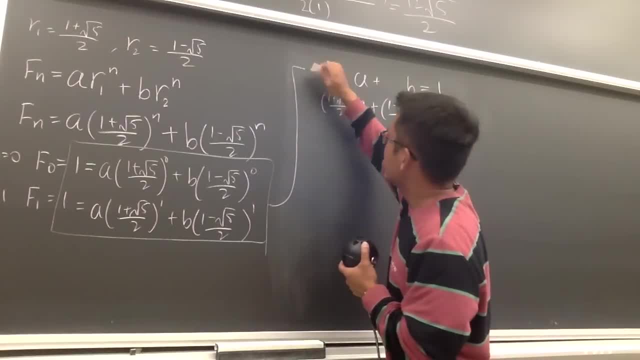 and this is equal to 1.. And if you look at this, I can say: let's eliminate A first And to do that we can just multiply the first equation by that. but negative of that, So negative, and let's put down parentheses around it. 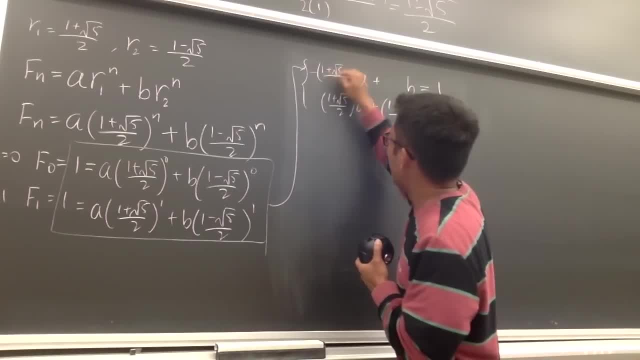 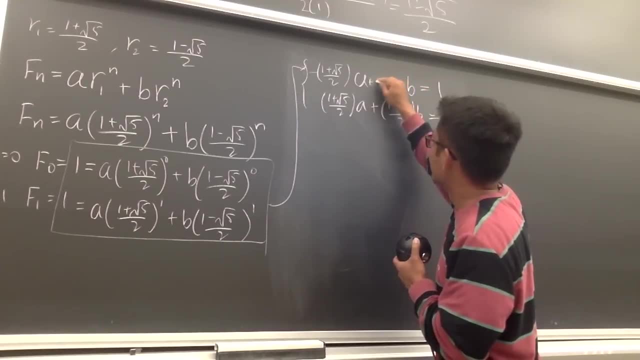 Negative parentheses: 1 plus square root of 5 over 2, and I'll put this down right here as well: Negative. so I'll just put down negative right here, and then 1 plus square root of 5 over 2,. 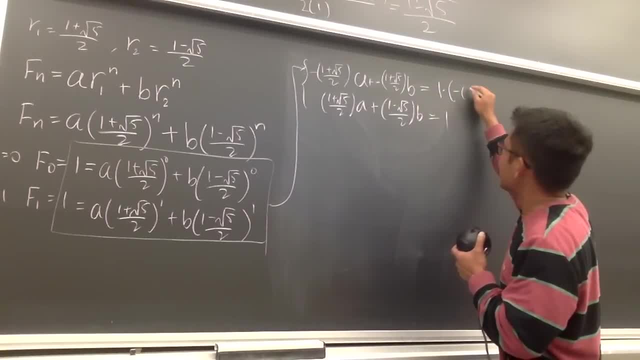 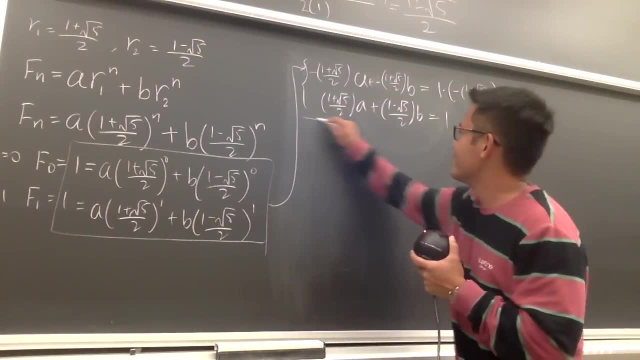 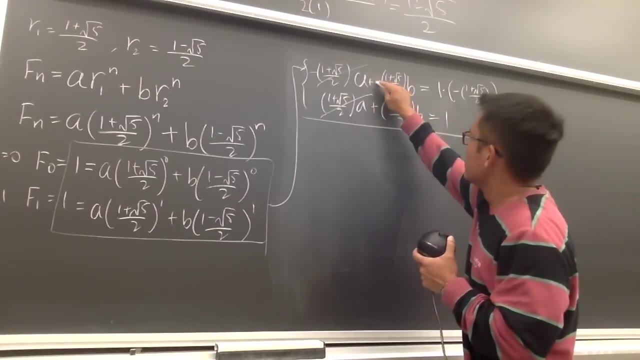 and at the end multiply by negative 1 plus square root of 5 over 2.. Like that right? Alright. So you see this and that will cancel each other out. This right here you have a negative in front. 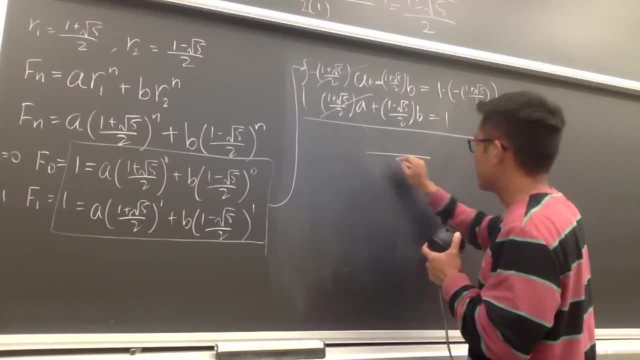 and they do have the same denominator, so I can put that down. on the bottom first right, You have negative 1 minus square root of 5, so let's put that down like this: After you distribute that, and then this is the positive version. 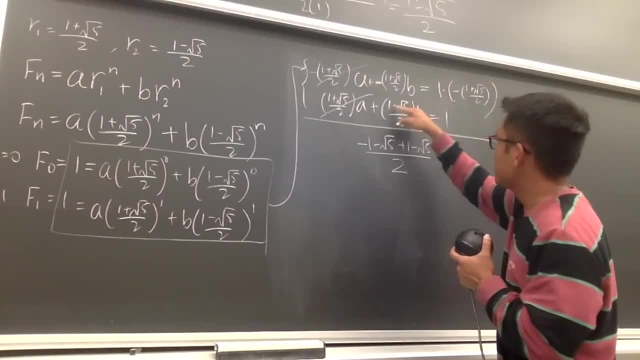 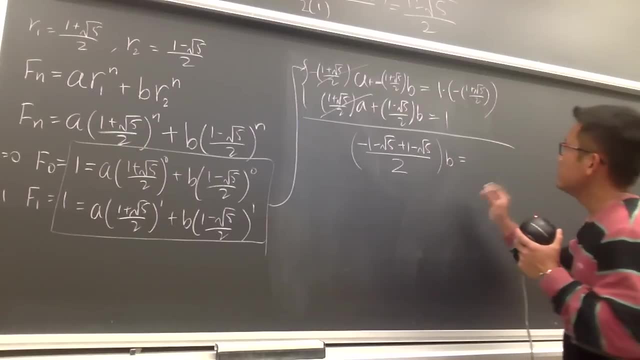 so you have plus 1, minus square root of 5, because that was originally a minus already, And this is, in parentheses- multiplied by b, and this is equal to the following: 1 is still 1, so let's put that down. 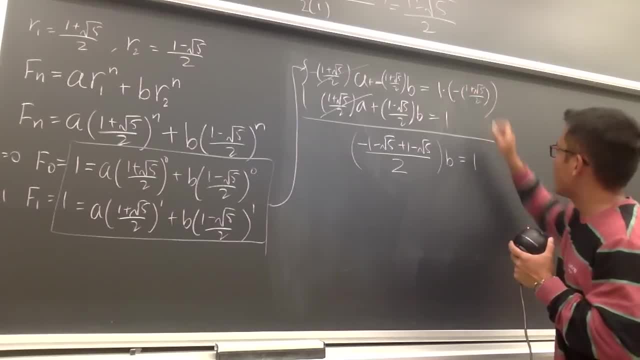 1 times. this is just that. but let me write it down as negative 1, and let's put the fraction separately, right? So negative 1 over 2.. I should put it down right here. And then negative square root of 5 over 2, right. 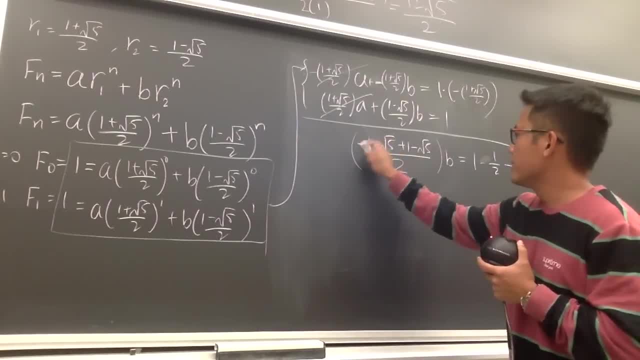 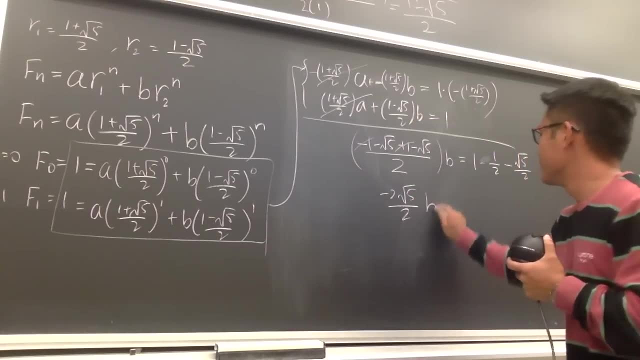 So just combine terms, Okay. So, as you can see right here: negative 1, negative 1, cancel Negative square root of 5, negative square root of 5, that's negative 2.. Square root of 5 over 2 times b. 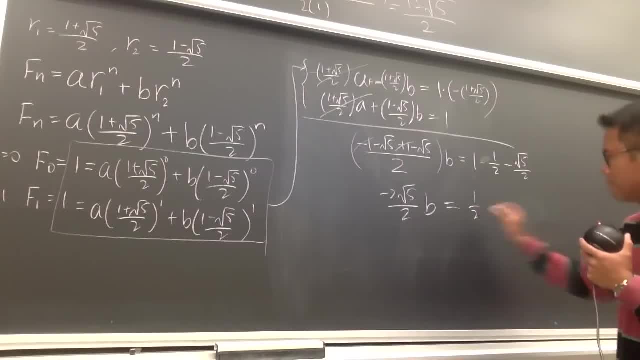 equals to 1 minus 1 half, just 1 half positive this time. And then we have the minus square root of 5 over 2.. And you see, this and that can be canceled, And of course b is going to be. 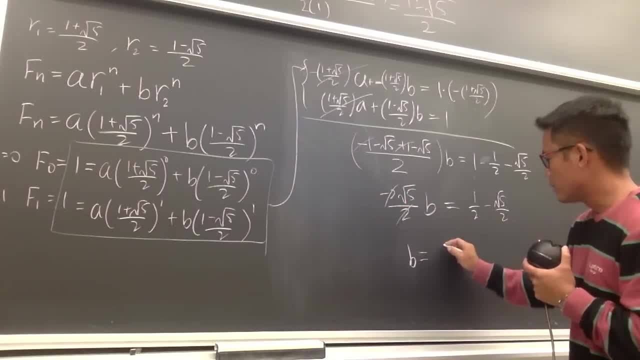 we can just divide both sides right by this number. So I would put that down like this: 1 over negative square root of 5.. And since they both have the same denominator, so I'll put this down right here. 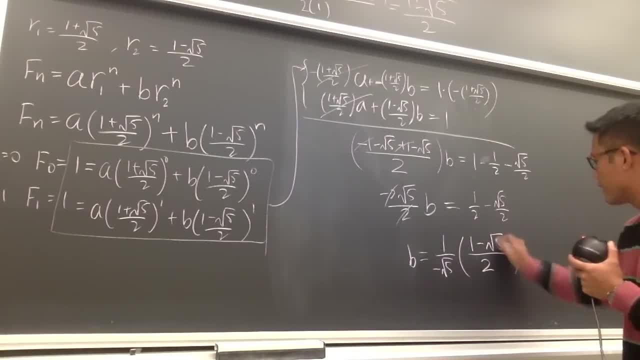 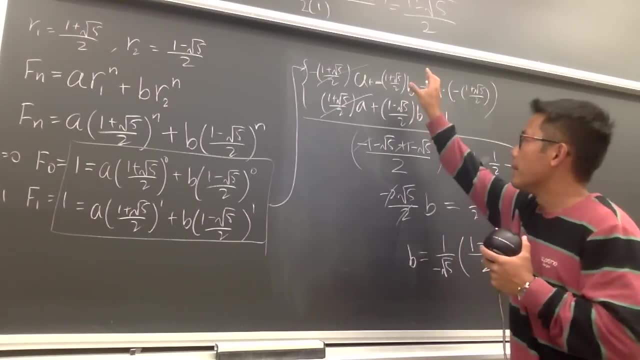 All over 2, on the top we have 1 minus square root of 5.. So this right here is the b value, And to get the a value, we pretty much do the same thing, but eliminate b instead, right. 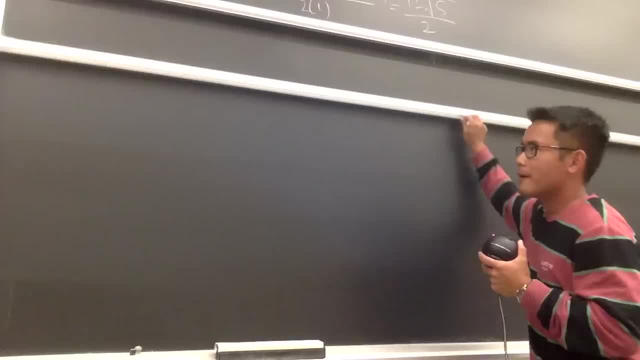 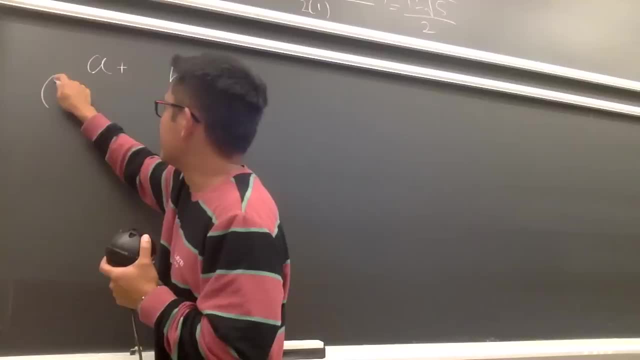 So I'll do that right here for you guys, because I have another board. So anyway, right here we know we have a plus b equals to 1. And a right here was with the 1 plus square root of 5 over 2.. 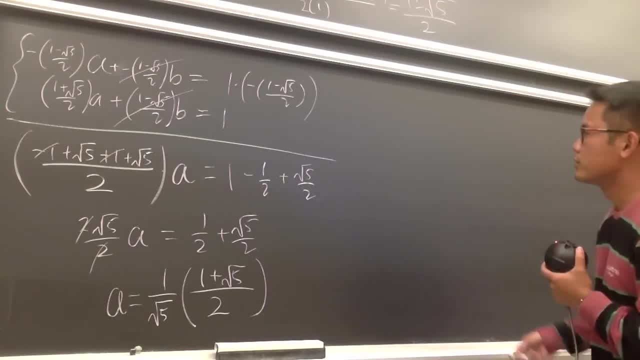 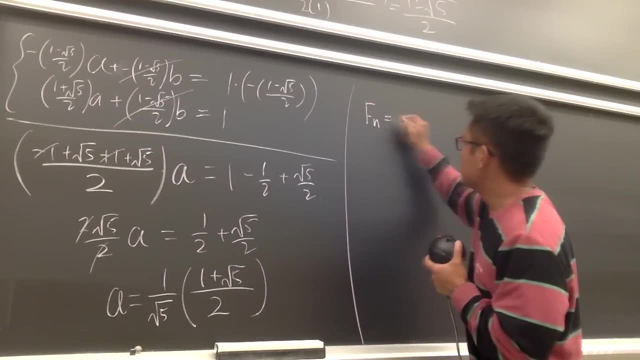 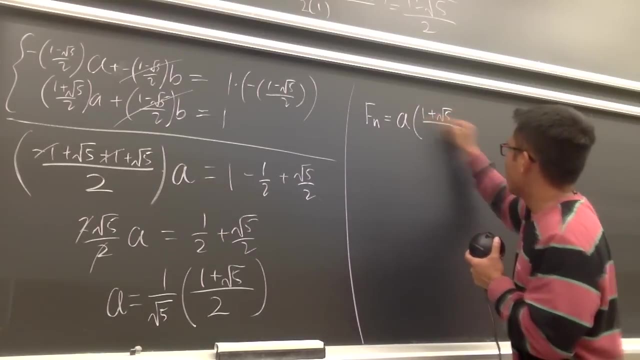 That, okay. So this is pretty much all we need. And now let me remind you guys: Fn- this is equal to a times something to the nth power, And this was R1.. R1 was 1 plus square root of 5 over 2 to the nth power. 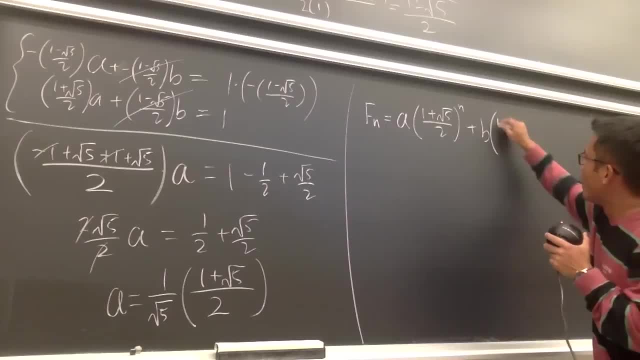 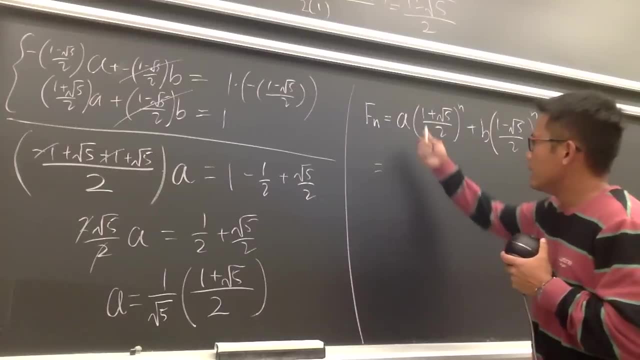 plus b times 1, minus square root of 5 over 2 to the nth power. And now we have the a b values already. a is this: So we see this is 1 over square root of 5 times this.